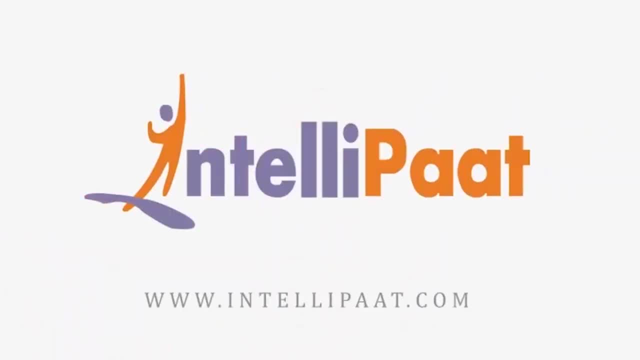 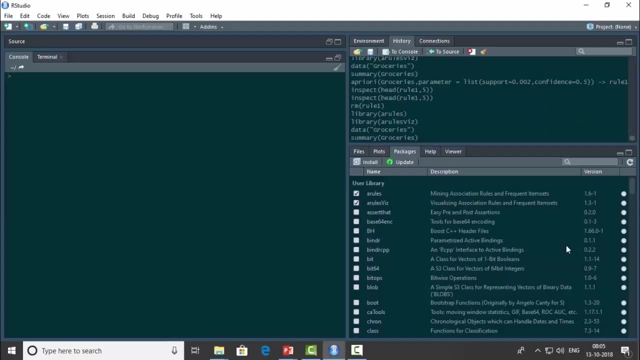 Alright, guys. so now we'll go ahead and implement the apriori algorithm in R. So this is R studio. and to implement the apriori algorithm, we are first supposed to load the arules package, So I'll type in library of arules and to visualize these association rules. we would also have 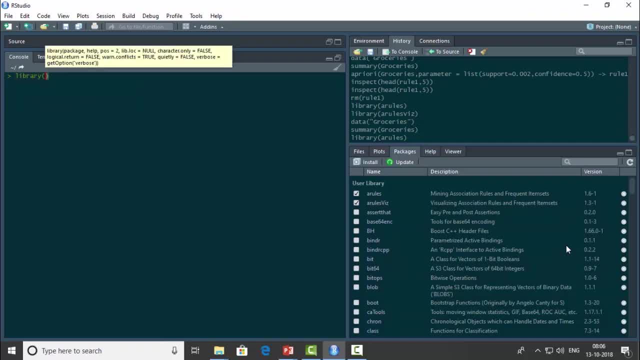 to load the arules vs package. So library of arules vs. So this arules package gives us a data set called as groceries. So let me load that. Now I'll have a glance at the summary of this data set. So, summary of groceries. So this is what we get. You see that these 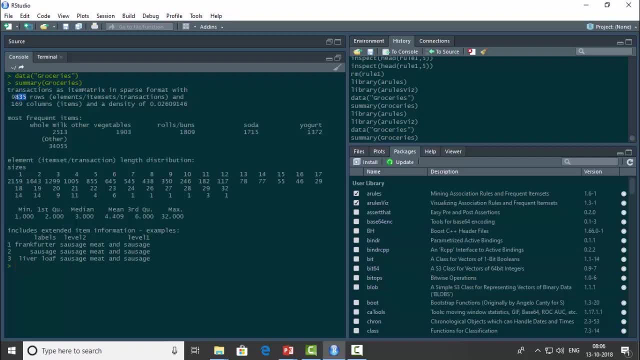 are transactions in the form of an item matrix and there are 9835 rows and 169 call levels, Or in other words, there are 9835 different transactions or orders and 169 different items. So we'll go ahead and find interesting relationships between these 169 different items And to 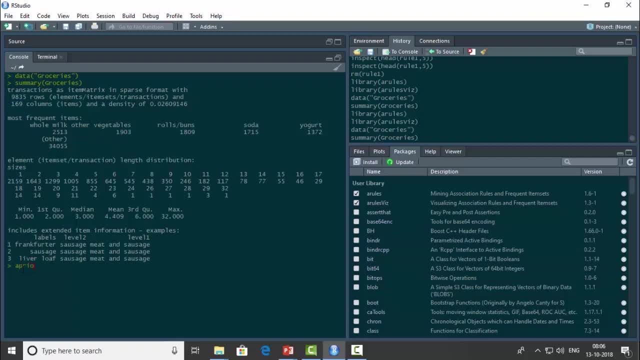 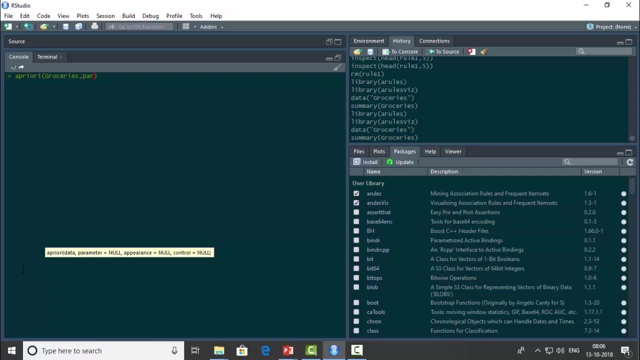 do that, we would have to load the apriori algorithm. So I'll type in apriori over here. So first I will give in the name of the data set, which will be groceries, and then I'll give in some parameters. So I'll type parameter over here. 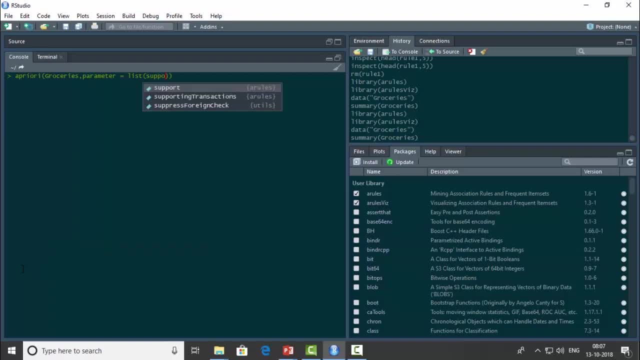 So I'll give some parameters, So I'll type parameter over here. So I'll type parameter over here So I'll give them the values for support, and confidence. So support, so the value which I give for support would be 0.002, and the value which 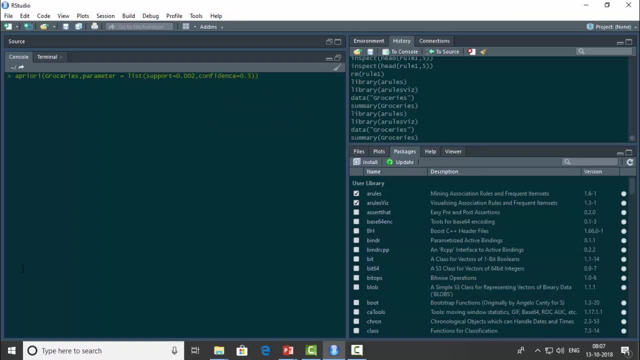 I give for confidence would be, let's say, 0.5.. So support basically tells us how significant is this rule. in the entire scheme of things, This value of 0.002 means 0.2%. of all the orders have the consequent and the antecedent. 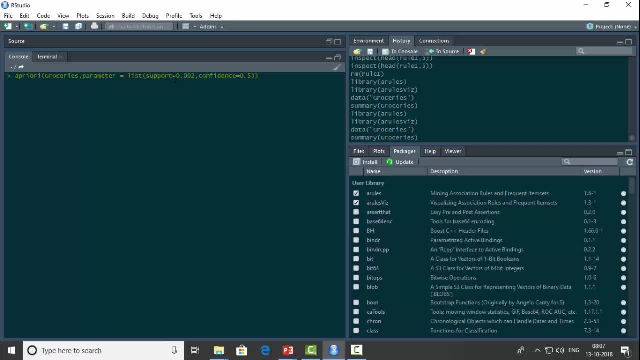 So 0.2% of all the orders have both the antecedent and the consequent. And this confidence value of 0.5 means that out of all the antecedents, there need to be at least 50% of them, which would also have the consequent. 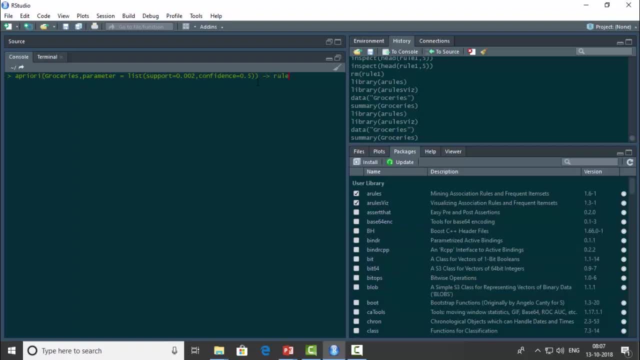 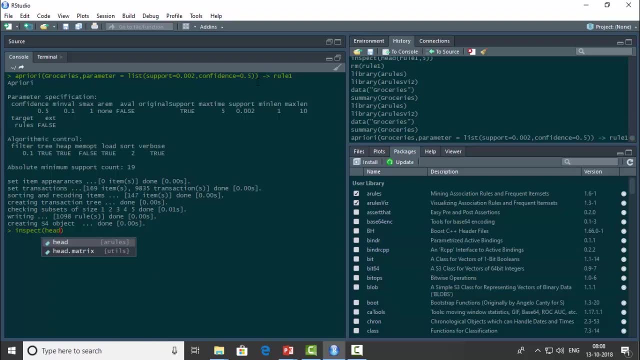 So now I will store this in, let's say, rule 1.. Now let me inspect these. inspect of. I'll type head and let me have a glance at the first five rules. So head of rule 1 and I'll type in 5 over here. 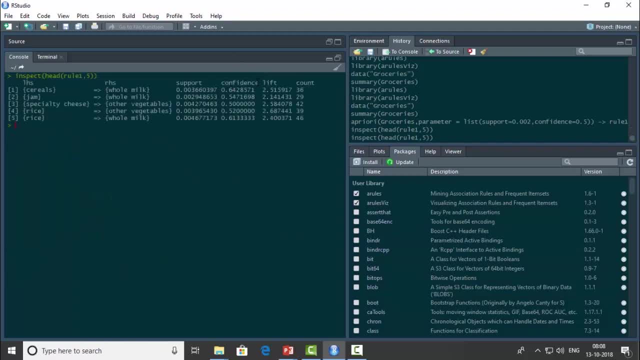 So, guys, this is what we get. Let me print this again. So these are the five rules which we get, And over here We also have the support value, the confidence value and the lift value. You see that if a person buys cereals, he is also likely to buy whole milk. 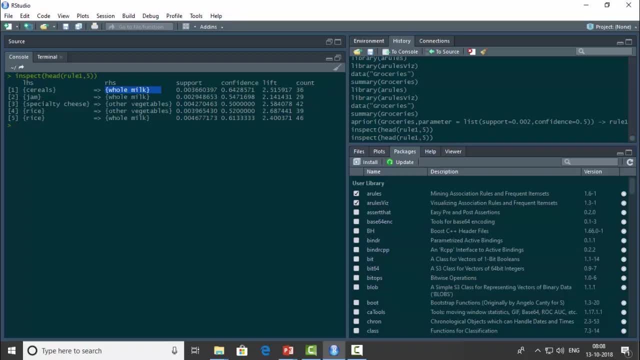 If he buys jam he is also likely to buy whole milk. So speciality cheese, other vegetables, rice, other vegetables, And again, if he buys rice, the consequent over here is milk. So these are the antecedents. 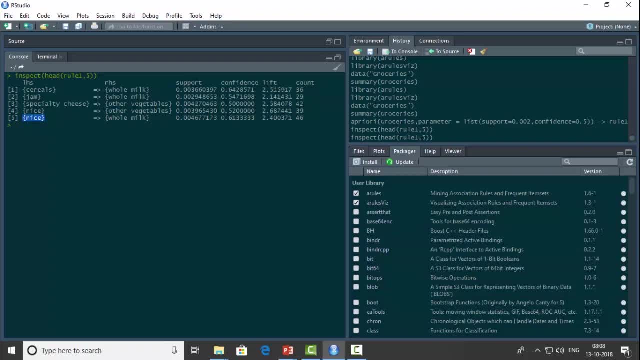 These are the consequence and these are the support value, confidence value and lift value. So again, let's understand the support value over here. The support value of 0.003 means that 0.3% of all the orders represent this LHS and RHS combination. 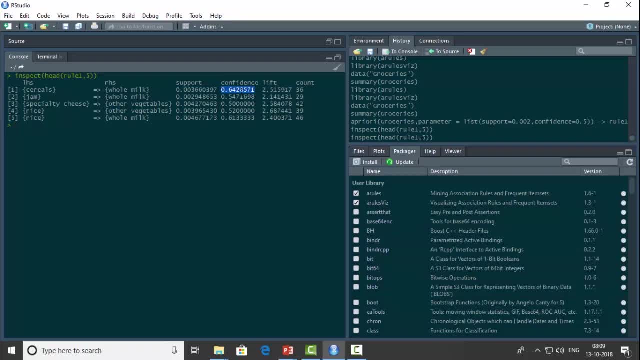 And again, this confidence value 0.64 means of the orders which contain cereals, 64% of them are likely to have whole milk. Okay. Similarly, again, the support value 0.002 means that out of all the orders, 0.2% of 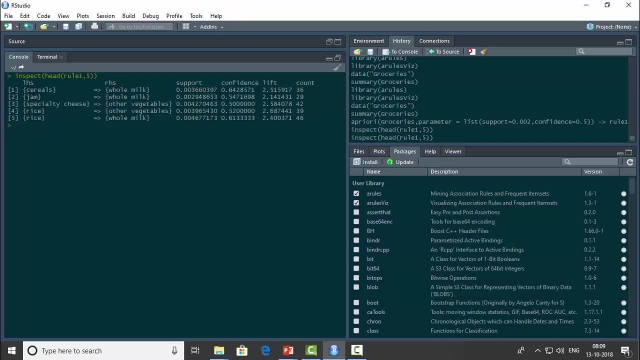 them represent this LHS and RHS Just combination, Okay, Okay, 0.54 means of the orders which contain jam, 54% of them would definitely contain whole milk. okay, so antecedent consequence, support value, confidence value and the lift value. so this lift value basically tell us how significant. 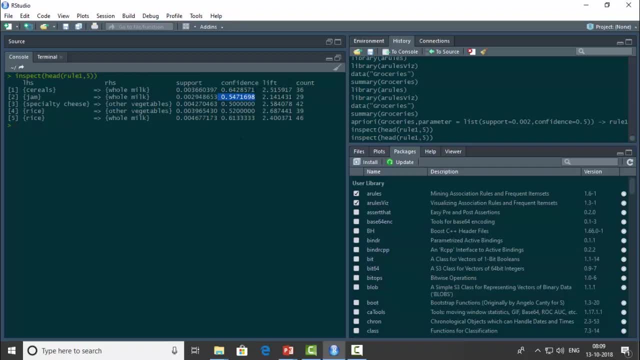 is the consequent with respect to the antecedent. so we see that this is like. all of these values are two times more significant, right? so now what I'll do is I'll sort them on the basis of lift- okay, so inspect head, sort of rule one- and I'll be sorting it on the basis of left. 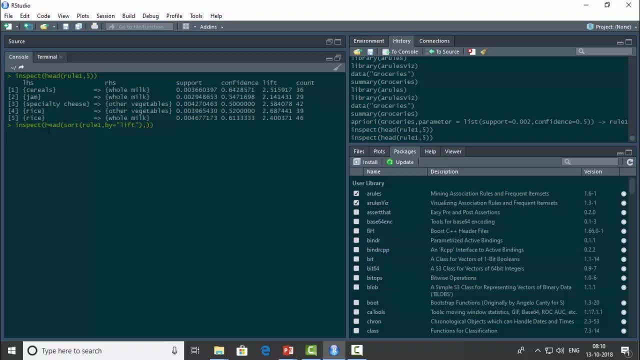 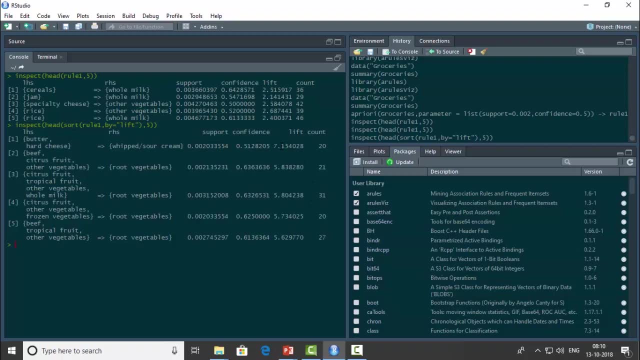 over here and let's see again. I do want to have a look at the first five rules. so this time these are lift values. so lift over here is seven, five, five, 5 and 5, and these are all the antecedents and these are all the. 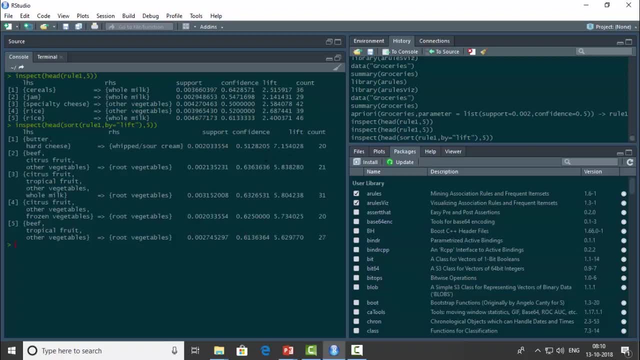 consequence, the support values and the confidence values over here to see that if the person buys butter and hard cheese, he is also likely to buy whipped or sour cream. similarly, if a person buys beef, citrus fruit and other vegetables, he's also likely to buy root vegetables again. if a person buys beef, tropical. 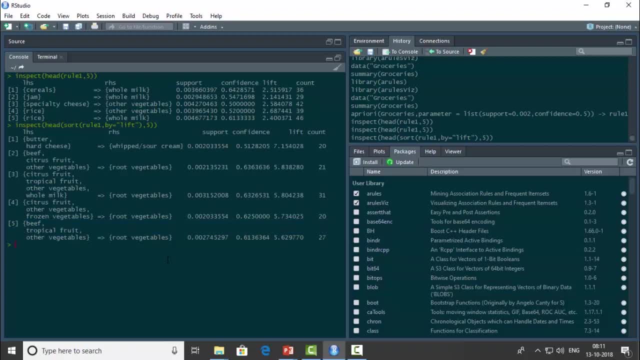 fruit and other vegetables. he is likely to buy root vegetables right, so now again. so the support value of 0.002 means that 0.2 percent of all the orders represent this LHS and RHS combination, and this confidence value of 0.51 means: 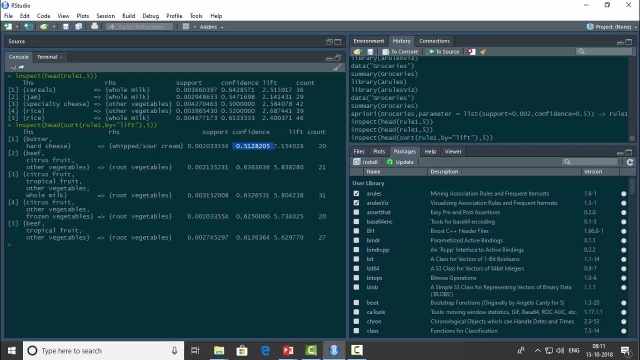 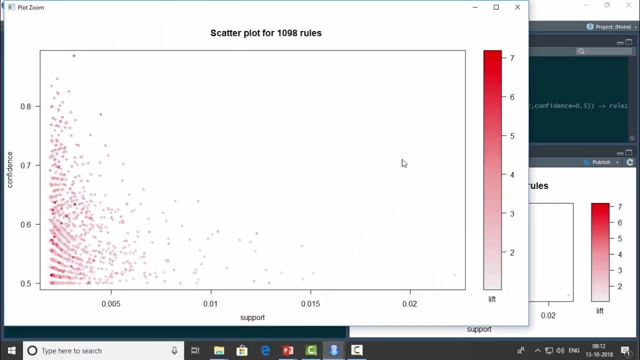 the orders that contain butter and hard cheese. 51% of them definitely contain whipped or sour cream. okay, now what we'll do is we'll actually plot these rules. so I'll type in plot of rule 1: So, guys, this is what we get over here. So let me zoom this first. 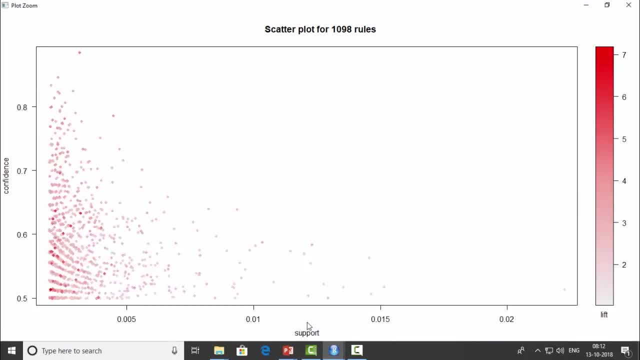 Right. so on the y-axis, we have confidence, on the x-axis we have support and this heat map which you see. so this is for the lift. So what you notice is these darker red dots are mostly occurring at low support values. So these 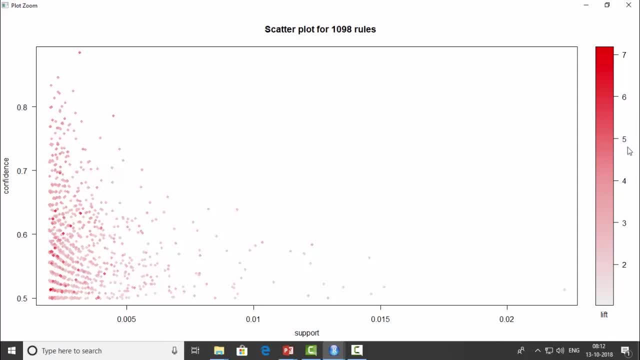 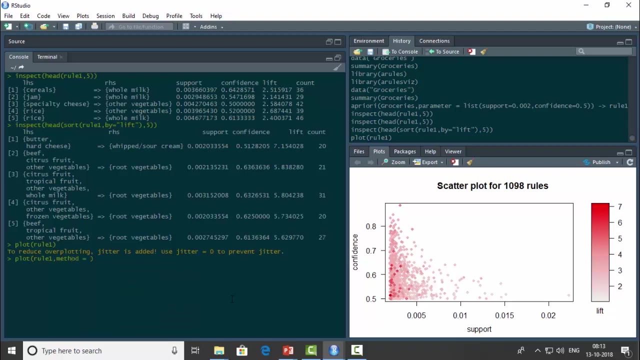 lifts, let's say 7x times, 6x times, 5x times- are usually prevalent when the rule itself is somewhat of an insignificant rule in overall scheme of things. So now we'll go ahead and plot this in a different way. So I'll give the method to be grouped over here and let's see what. 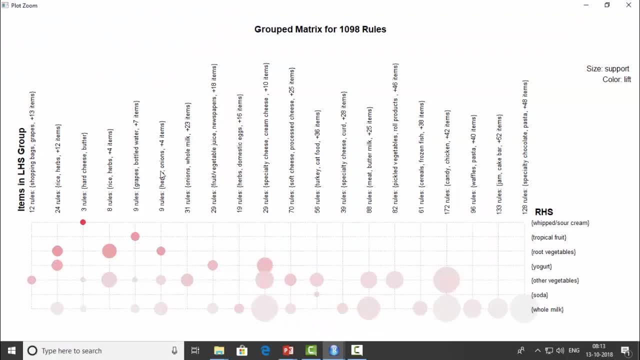 do we get Right. so this time this is what we get. So these are all the items in the LHS group and these are all the items in the RHS group. So over here, the size of the bubble represents support and the color of the bubble represents lift. so what you? 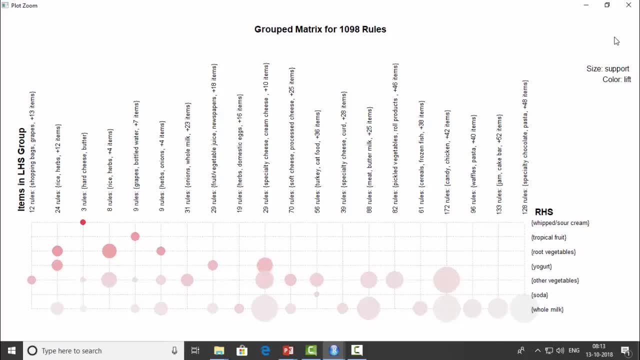 notice is: larger the bubble, greater is the support and darker the bubble, greater is the lift. so let's say we would want to find a compromise between the support and the lift. then this or this one would be an ideal value. so let's see. so this is the rule over here. so the antecedent is rice, herbs and four. 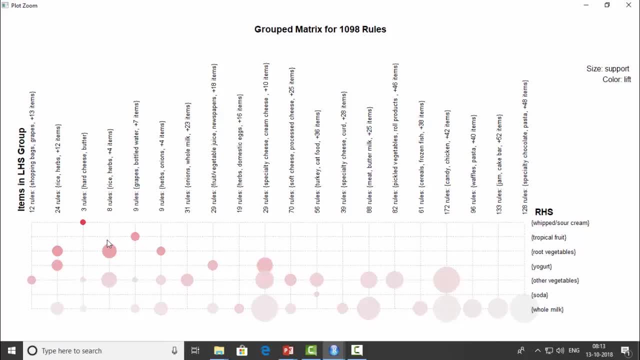 other items and the consequent is root vegetables. so there is a proper compromise between support and lift over here. similarly, we can also take- let's see this value over here. so over here this is rice herbs and 12 other items and again the consequent over here again is root vegetables. right, so this was one. 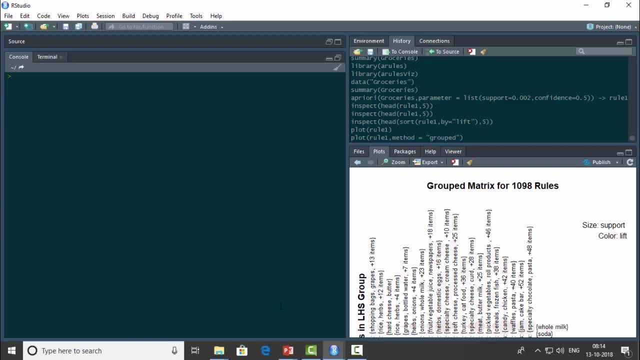 rule which we built. now we'll go ahead and change the parameters and get another set of rules. so again, let me build the a priori algorithm. I'll give in the data set, which is groceries over here, I'll give in the parameters, so it'll be list again. 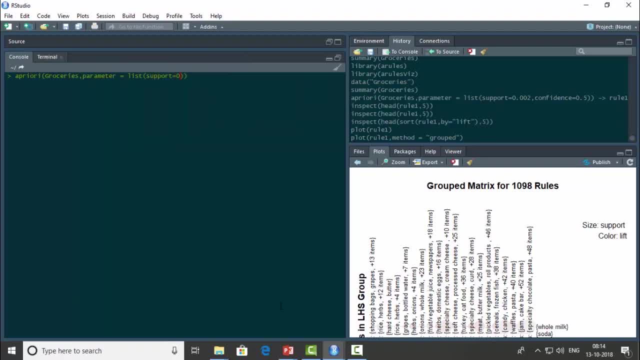 the support value which I'd be giving would be 0.002 and the confidence value which I give 0.5. now, coming to the antecedents, I would want a minimum length of at least five minutes. okay, so I'll say min len equals five and I will store this in rule two. so let 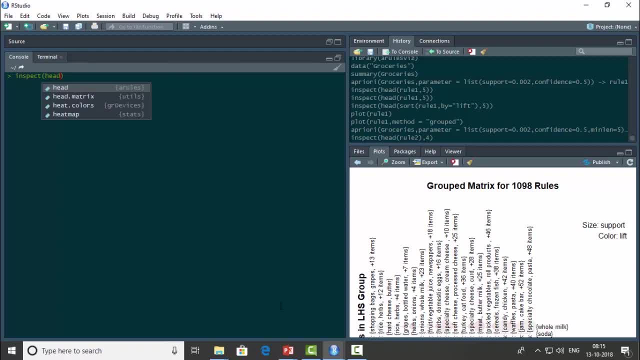 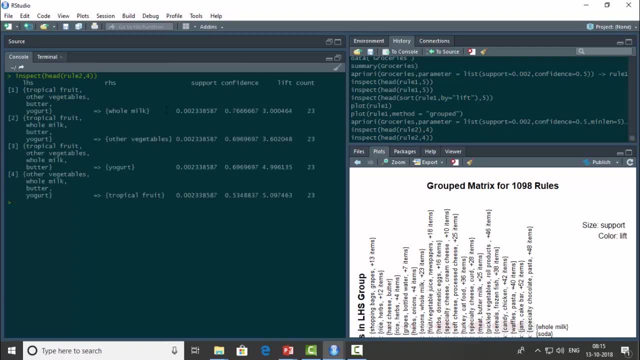 me inspect this. so inspect of head. I'll type in rule two and I don't want to have a glance. the first four rules, right? so we see over here that the minimum length for all of these is five. so the empty set is also counted as one. 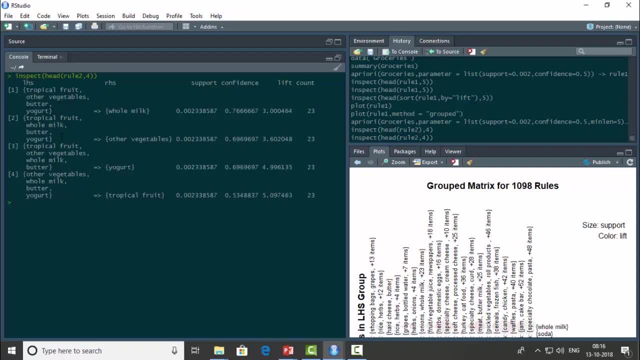 item. so one, two, three, four plus the empty set makes it five again. one, two, three, four plus one makes it five, four plus one, five, four plus one, five. so over here the antecedents are tropical fruit, other vegetables, butter and yogurt and the consequent is whole milk. over here again the antecedents are tropical fruit. 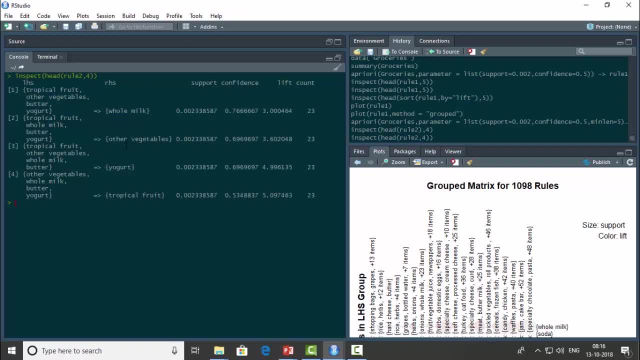 whole milk, butter and yogurt, and the consequent is other vegetables. similarly, for this, the antecedents are other vegetables, whole milk, butter and yogurt, and the consequent is tropical fruit. and for these, these are the support, confidence and lift values. so let's examine this. the support value is 0.002. 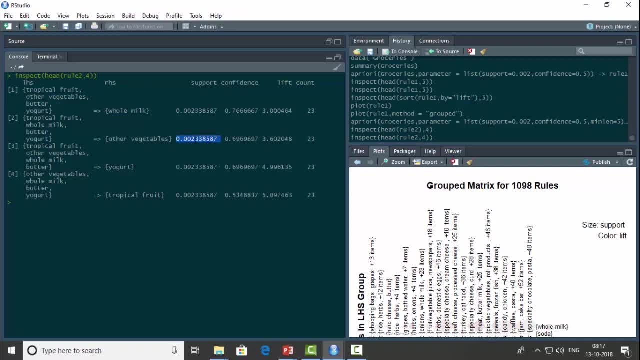 and this means that there are 0.2% of all the orders which represent this LHS and RHS combination right and again a confidence value of 0.69. this means that out of all the orders which contain tropical fruit, whole milk, butter and yogurt, 69% of them would definitely contain other vegetables. now let me 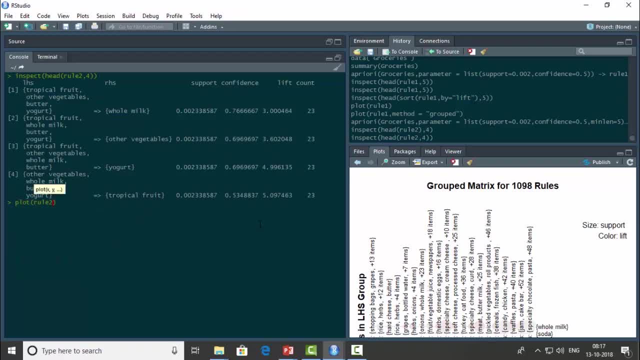 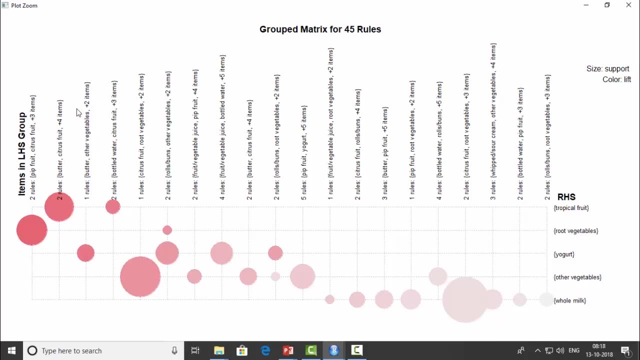 also plot these. so plot of rule 2 and I will group them. method equals grouped. so this time this is what we get over here. so LHS are the antecedents, RHS are the consequence and again, size over here represents the support value to the product type LHS. 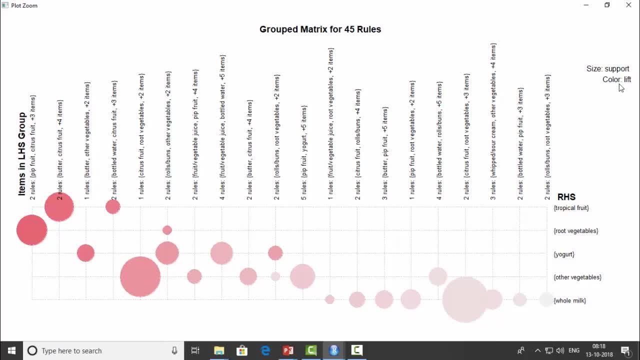 and color of the bubble represents the left. So it's the same thing. So larger the bubble, greater is the support, Darker the color, greater is the left, and we'd have to find a compromise between the support and the left, So these two seem. 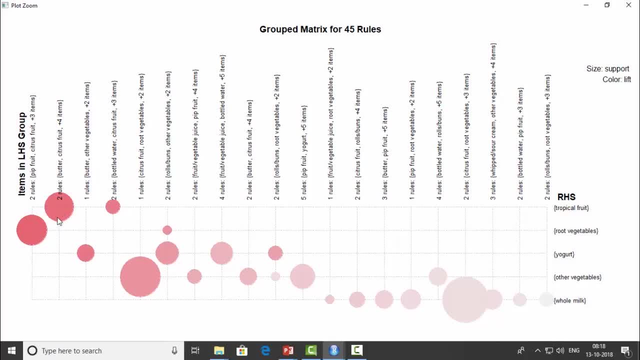 to be the ideal values over here. The bubble size is also big and the color is also dark, So for this it has a pip fruit plus citrus fruit and three other items, and the consequent is root vegetables, And for this it's butter plus citrus. 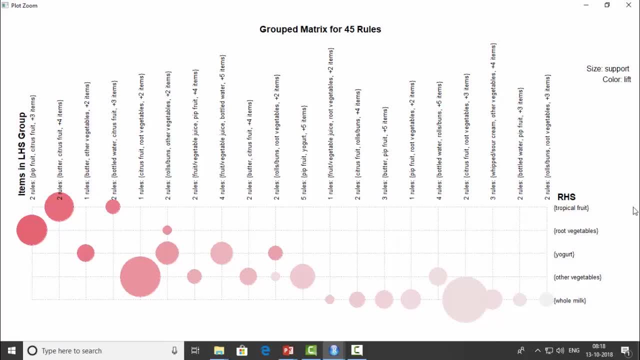 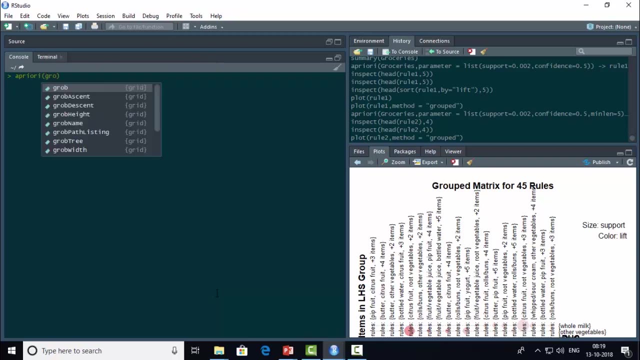 fruit and four other items, and the consequent is tropical fruit. again Also, this seems to be good. It's rolls or buns. other vegetables, two other items and the consequent is yogurt. Okay, now we'll build another rule, So it'll be apriori. Let me give in the name of the data set, which would be: 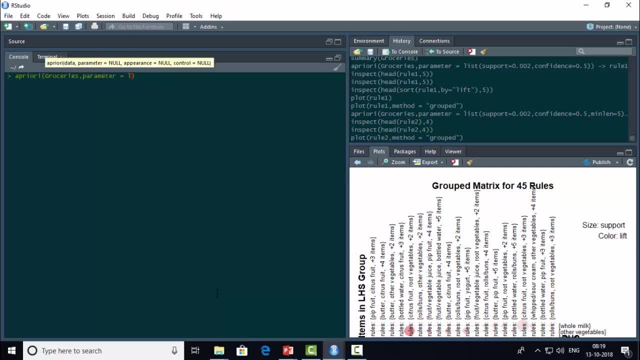 groceries. After this I'll give it the parameter, I'll type list over here and this time I'll change the values for support and corn confidence. so the support value which I'm giving is 0.007 and the confidence value which I'm giving would be 0.6. okay, so this means that 0.7% of all the orders would have both. 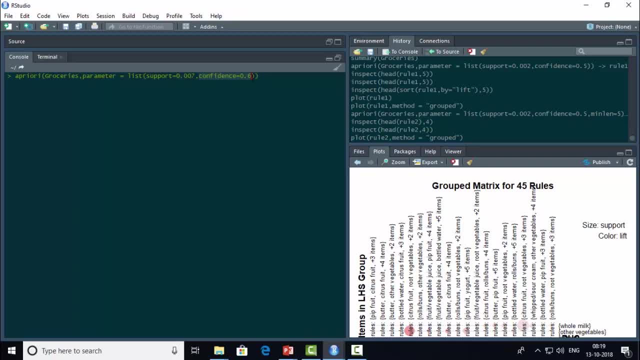 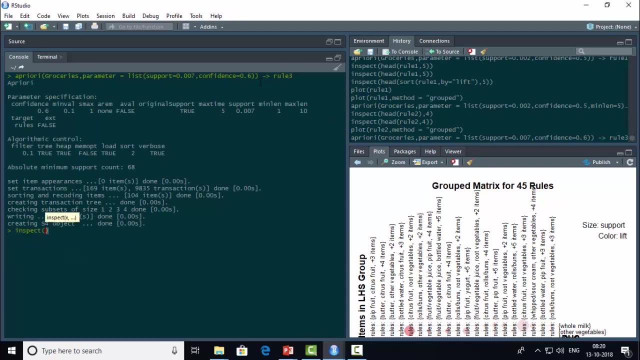 the antecedents and the consequence. and the 0.6 value means that out of all the antecedents, at least 60% of them would definitely have the consequent. so I will store this in rule 3. let me inspect this inspect of head. I will give in the rule which is rule 3, and again. 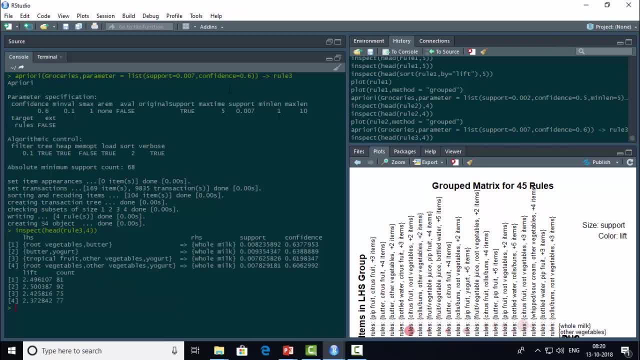 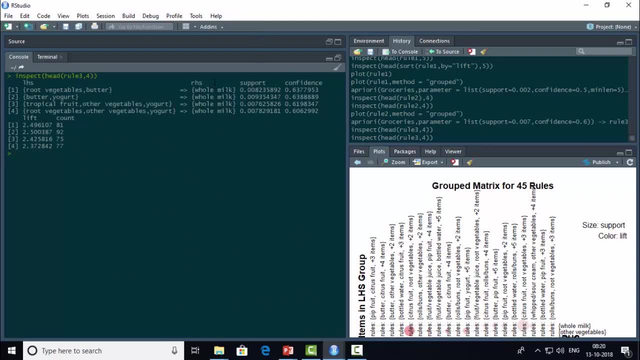 I do want to have a glance of the first four rules. so this is what we get over here, right? so these are the antecedents and these are the consequences, and we see that for all four the consequent is just milk. so if a person buys root vegetables, 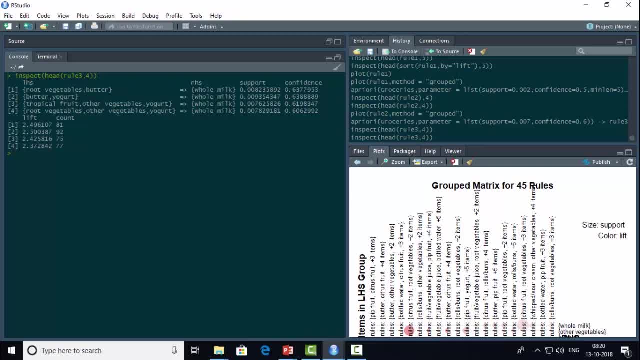 and butter, he's also likely to buy whole milk. if a person buys butter and yogurt, he's also likely to buy whole milk. similarly, if a person buys root vegetables, other vegetables and yogurt, he's also likely to buy whole milk. and these are the support and confidence values. 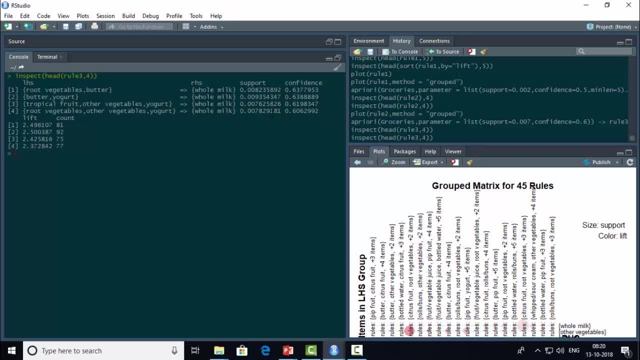 over here. so the support value for this one is 0.007 and the confidence value is 0.6. this value 0.007 means that 0.7% of all the orders represent this LHS and RHS combination, and this value of 0.6 means that of the orders which contain root vegetables, other vegetables. 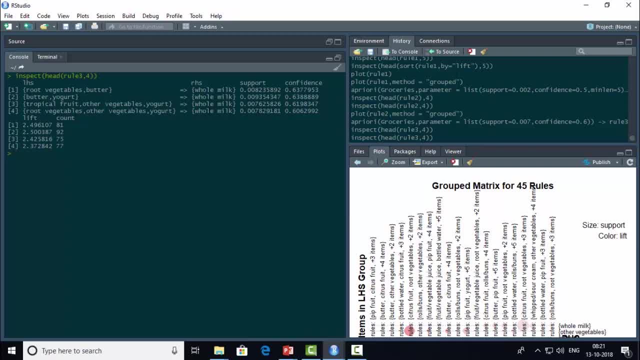 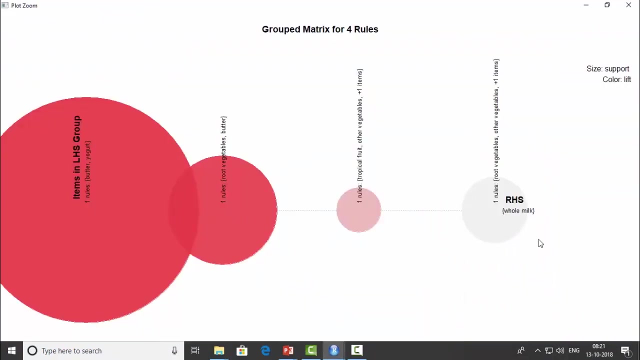 and yogurt. 60% of them would definitely contain whole milk. again let me plot this plot of rule 3, and again the method would be grouped right. so this time we just have four bubbles over here, so there seems to be our ideal value. so this is the darkest and the size of the bubble is also the highest. so over here, the